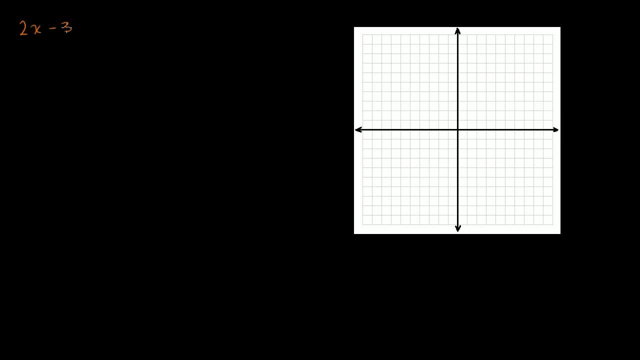 Let's say we have 2x minus 3y is less than or equal to 21.. And we've seen how to graph this before. You can just graph this line and then figure out what the less than part means. So let's just rearrange this into slope intercept form. 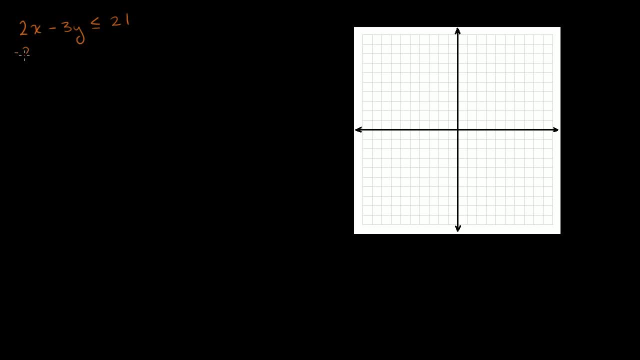 So if you subtract 2x from both sides minus 2x, subtract 2x from both sides, we get negative 3y. these cancel out is less than or equal to 21 minus 2x, or we could say negative 2x plus 21.. And then we can divide both sides by negative 3.. 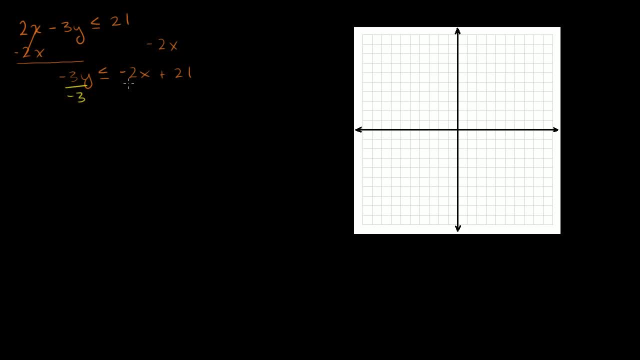 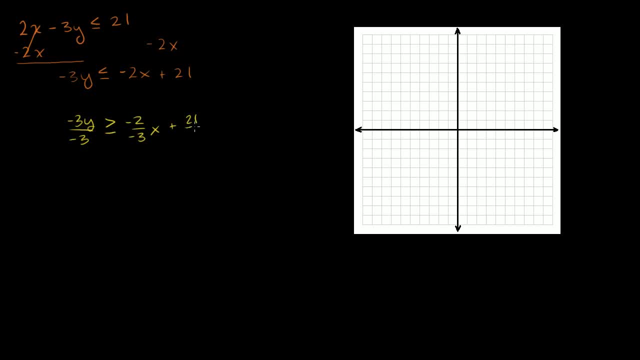 So you get negative 3y over negative 3x plus 21 over negative 3.. And so this equation becomes: y is greater than or equal to 2 thirds x minus 7.. So that's this first inequality. right there, Let's graph it. I'll graph it in orange. 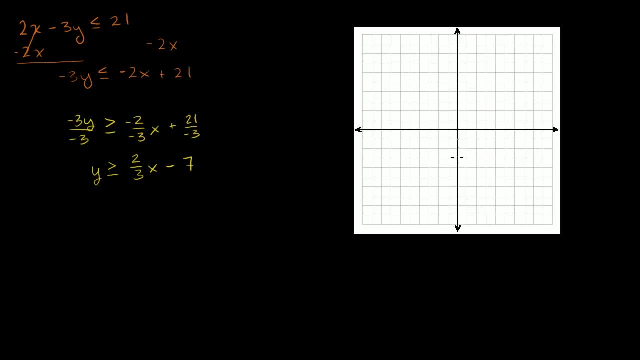 y intercept is negative, 7.. So 1,, 2,, 3,, 4,, 5,, 6,, 7.. And its slope is positive 2 thirds. So when you run 3,, you go up 2.. 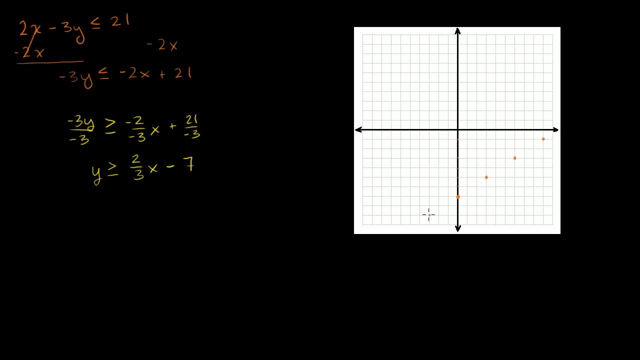 And in this direction, if you go back 3,, you go down 2.. So the line will look something like this. The line will look like that: Keep going. And since we have y is greater than or equal to, essentially this line, the area that satisfies the line is negative. 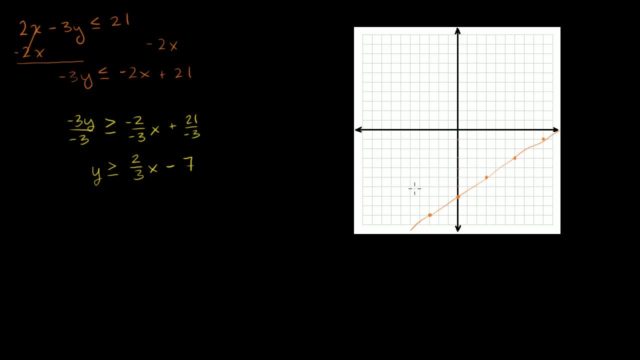 Because this inequality is going to be above the line At any point. for any x, for any x you pick, this is the value 2 thirds x minus 7.. So if y is going to be greater than that, it will be all of the points above that. 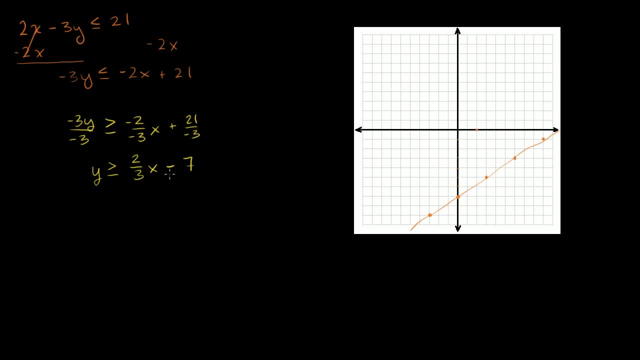 So just this constraint right here: y is greater than 2 thirds x minus 7, or this constraint, which is the same thing: 2x minus 3y is less than or equal to 21.. We'll give you all of this area up here. I don't want to draw it too dark just yet. 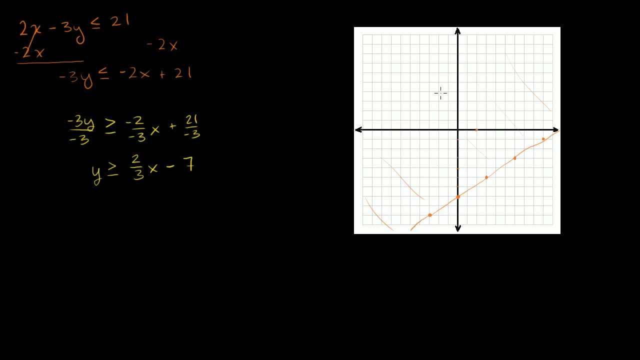 So we'll give you all of this area all the way above this line. Now let's add another inequality to the mix. Let me do that other inequality in blue. Let's say I have x plus 4y. Let's make it less than 6.. 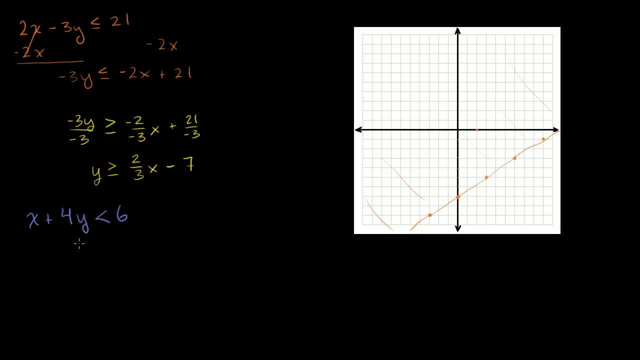 The problem I have written here is less than or equal to, But I want to mix it up with an equal sign and a couple of them without an equal sign, Just so we remember how to graph these things. And so let's put this again. 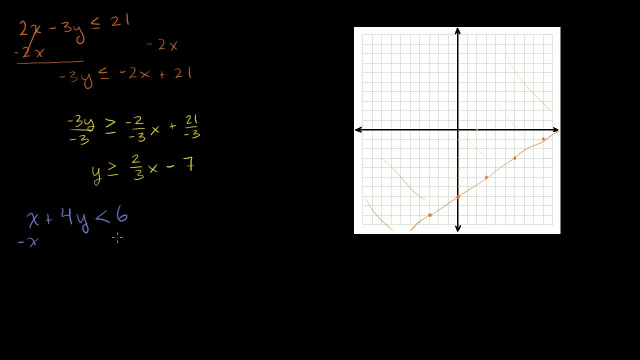 Let's put this into slope intercept form, So we can subtract x from both sides. Then the left hand side just becomes 4y, The right hand side becomes negative x plus 6. And then we can divide both sides by 4.. 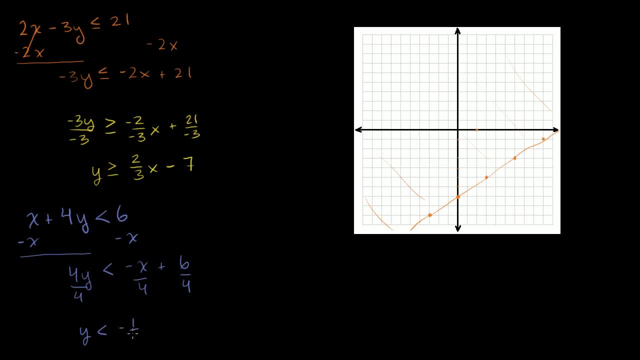 And we get: y is less than negative, 1, fourth x plus 6.. So, just like the first equation, let's graph the line. The line is: The y intercept is positive, 6.. So 1,, 2,, 3,, 4,, 5,, 6.. 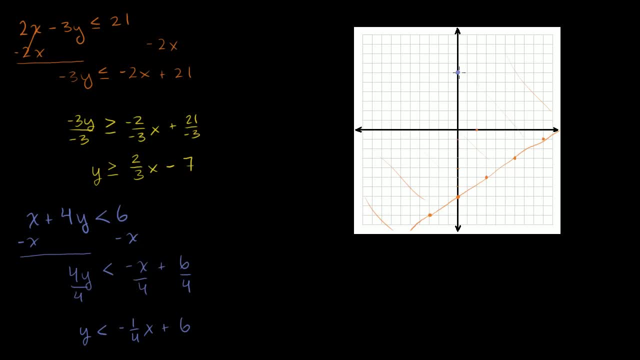 And then the slope is negative 1. fourth: So every time we run by 4, 1,, 2,, 3,, 4, we're going to go down 1.. So you run by 4, 1,, 2,, 3,, 4, you go down 1.. 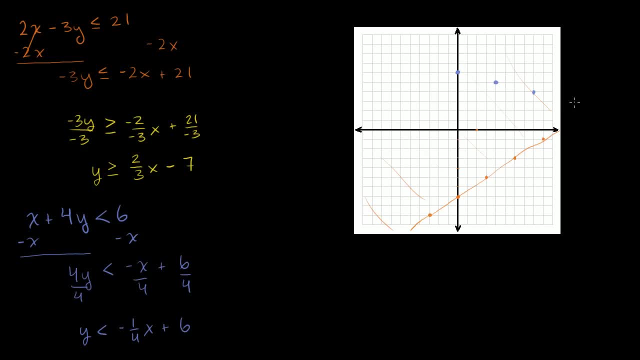 You run by 4,, 1,, 2,, 3,, 4,, you're going to go down 1.. So this line is actually going off the table. If you go back by 4,, 1,, 2,, 3,, 4,, you're going to go up by 1.. 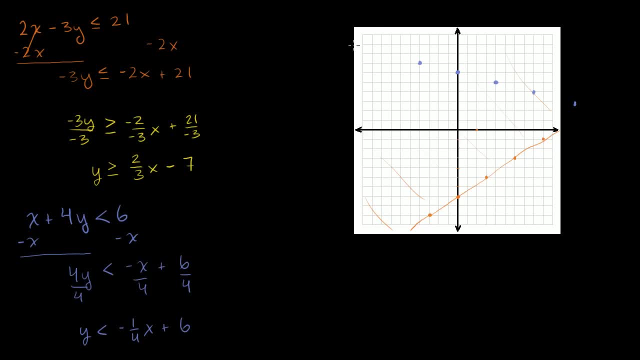 1. 1. 1,, 2. Actually including the line we're going to have to draw a dotted line here. So it's going to be a dotted line. I'll draw my best. I'll try my best to draw a dotted line. 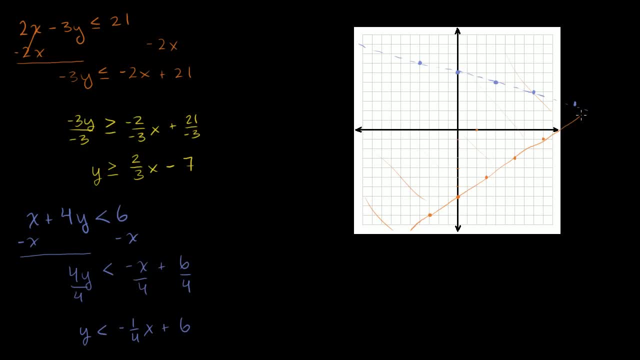 Actually let me continue that previous line there because I actually want to show where the intersect goes a little bit off of our graph paper. But the graph of this equation is that, right there, I did a dotted line because it's not less than or equal to: 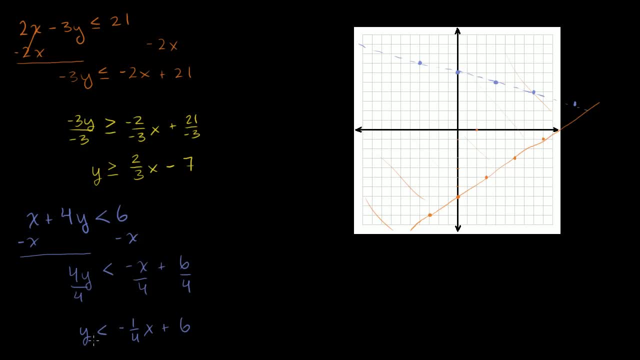 It's just less than So. this inequality, if I were to graph it, it would be the area below the line, It would be the area below the line, The area below the line right there. That's what satisfies this inequality For any x. this is the value of that line, but the y's that. 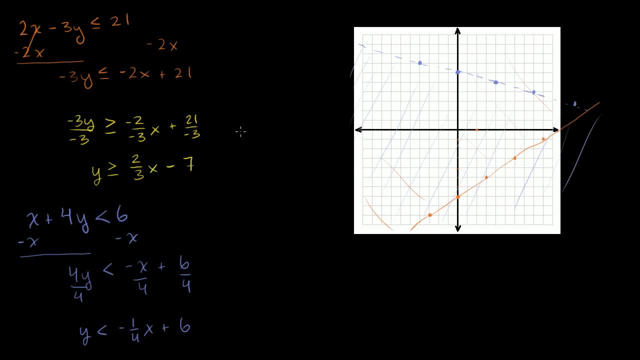 satisfy, it are the y's that are below the line. Now, if I were to ask you if I were to have a system where I have 2x minus 3y is less than or equal to 21, and another equation or inequality, I should say: 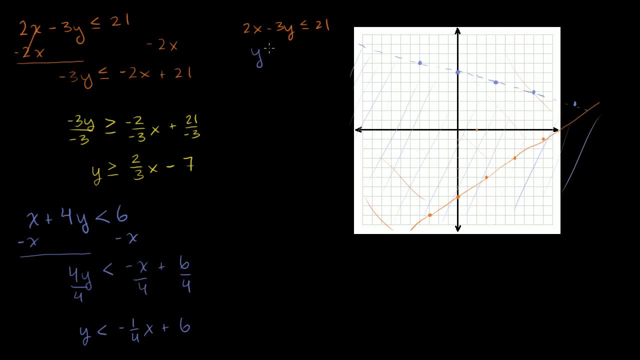 These aren't equations, These are inequalities. They're not equal to each other. The other one is: x plus 4y is less than 6.. And if I were to ask you what x's and y's satisfy, both of these inequalities, well you'd say: well, gee, it's. 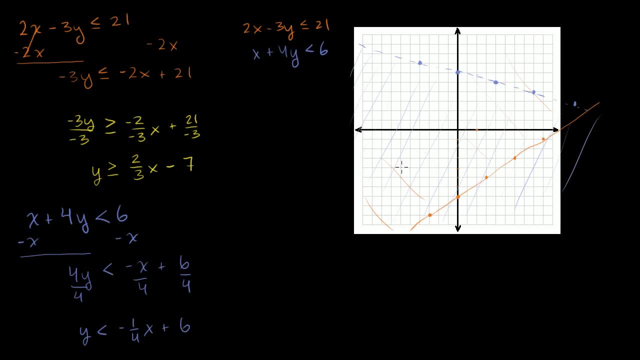 just going to be the overlap of their solution sets. It's going to be the area in the xy plane that satisfies both of them. So in this case it'll be the part that's above the orange line. Remember, I shaded that in orange, right there. 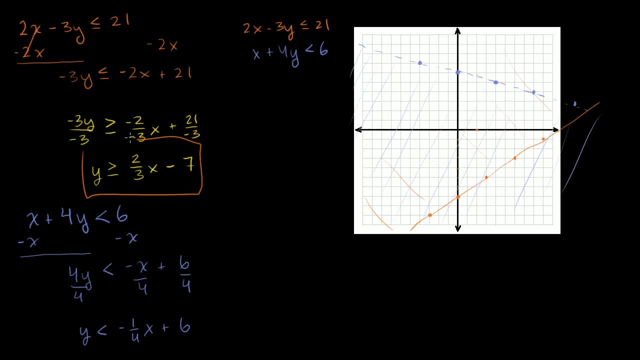 The part that's above the orange line. That's that right there. So all of this above the orange line and the part that's below the blue line And the part that overlaps, that satisfies both of these. I'll do it in yellow. 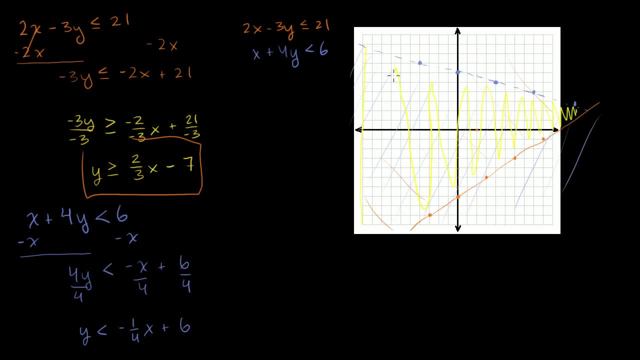 The part that satisfies both of these is right in between the lines there. Now what if, just for fun, we were to add a third equation? Let's add a third equation: in green, 3x plus y is greater than or equal to negative 4.. 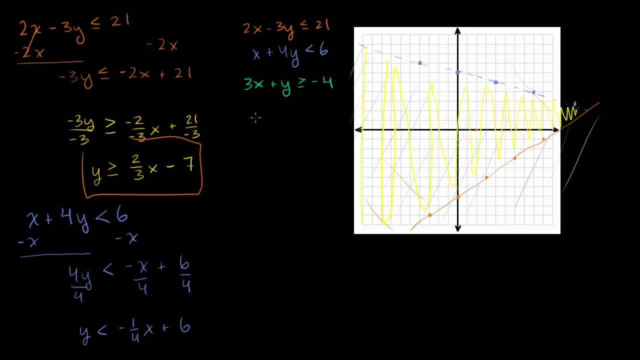 Well, it's the same drill. We put this in a slope-intercept form, So you get: y is greater than or equal to negative 3x minus 4.. I just subtracted 3x from both sides. We can graph this line: 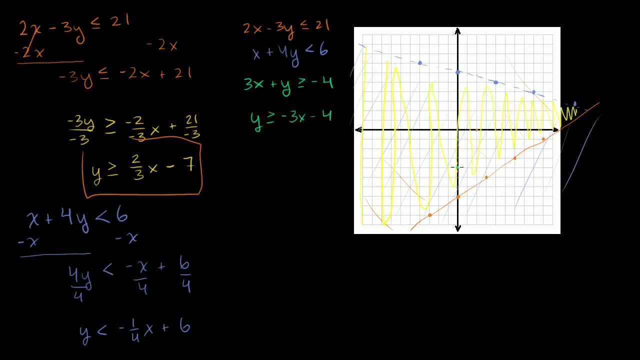 Its y-intercept is 1,, 2,, 3,, negative, 4. And it has a slope of negative 3.. So every time you go 1 to the right, you go down 3.. 1,, 2,, 3.. 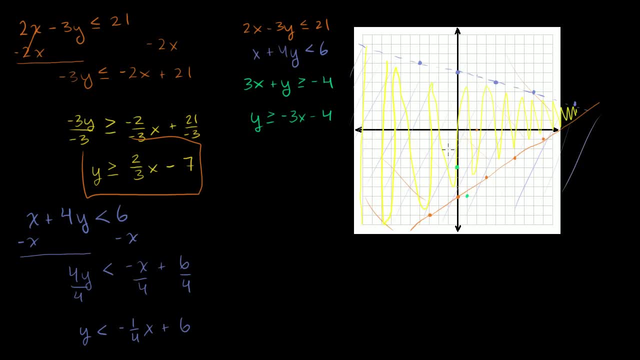 If you go 1 to the left, if you go negative 1 in the x direction, you go up 3.. So you go Negative 1, 1, 2, 3.. Negative 1, 1, 2, 3.. 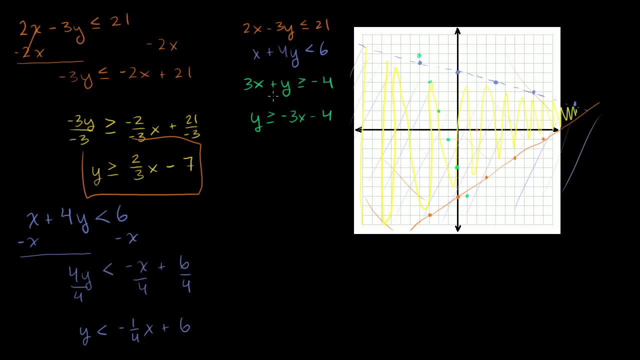 Negative: 1,, 1,, 2,, 3.. So this line right here, this line right there, is going to look like this. It's going to look like that: Trying my best to draw it. That's that, right there. 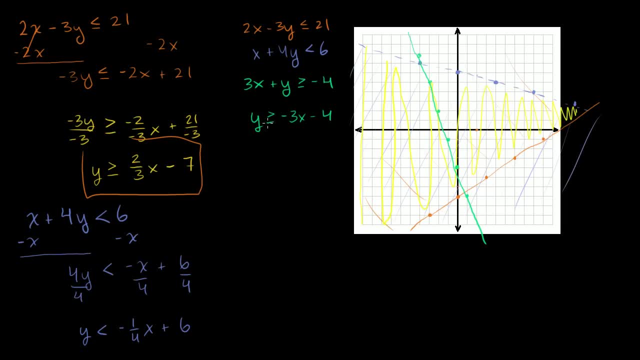 And I can have it in bold. I don't have to do a dotted line because I have a greater than or equal to. And so what are all the y's that are greater than this line? Well, for any x value, you pick the value of negative 3x. 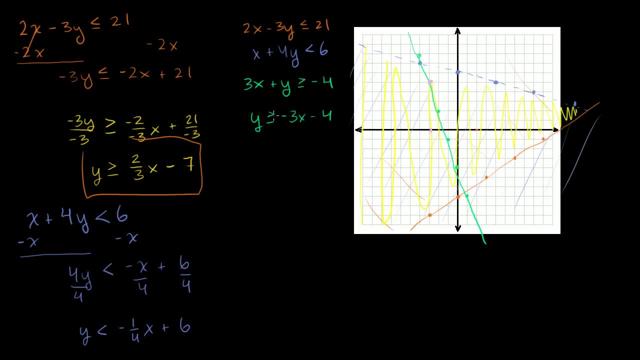 plus negative 3x minus 4 is going to be this, And we care about the y values that are greater than that, So it'll be above the line. So for just this inequality it'll be everything above the line. And then if someone were to come along and say: 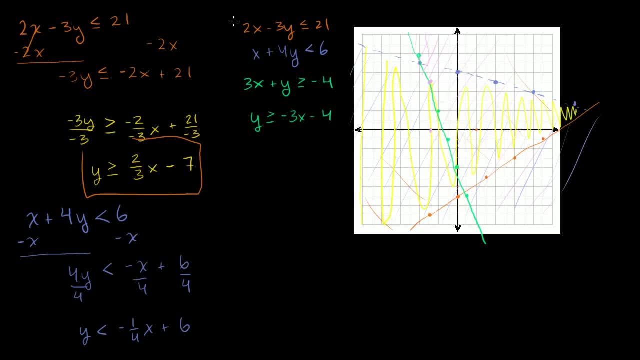 all right, tell me, show me, graph me all of the points on the xy plane that satisfy this system of inequalities. what would you tell them? Well, it would be the overlap of their solution sets So the part of the xy plane that exists in all. 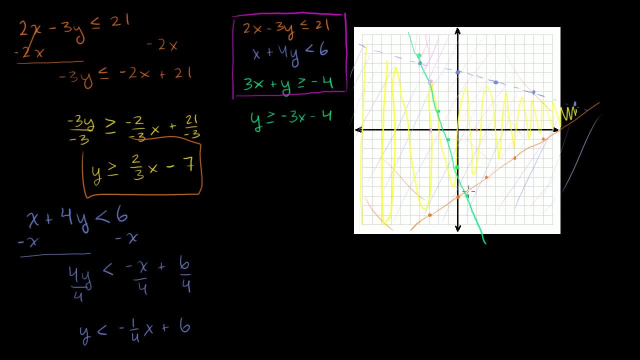 of their solution sets. So it's above the orange line. We have to be above the orange line. We graphed that before. It was all in orange before, because we're above the line 2x, 2 thirds x minus 7.. 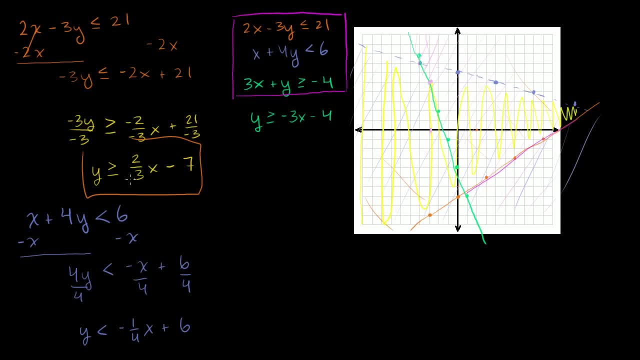 It might trick you a little bit because it has a less than here, but when you put it in the slope-intercept form you have a greater than So. it's everything above this line, which was all of that over there, Everything below this line, below the blue line.